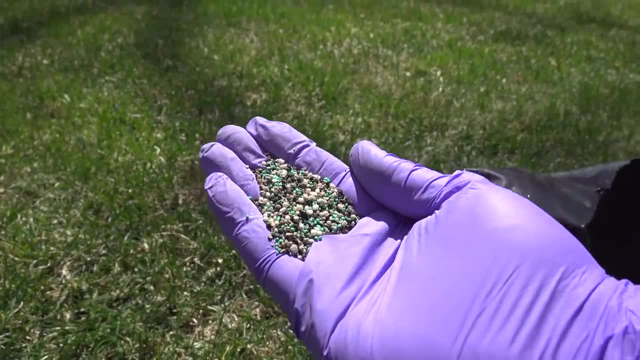 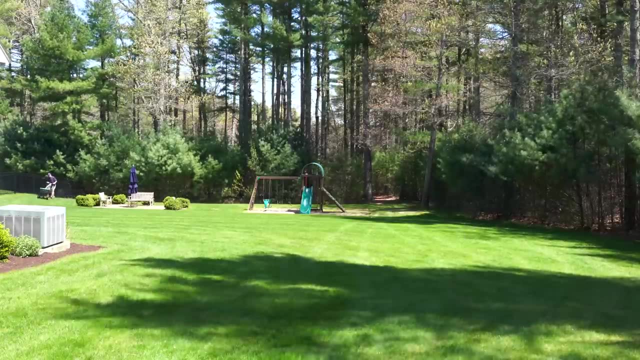 And I don't blame them for being confused, because there are so many new fertilizer companies on the market. Most of these companies go out of business within a few years because their products don't really deliver results. Now, lawn fertilizers are a lot simpler than you might think. 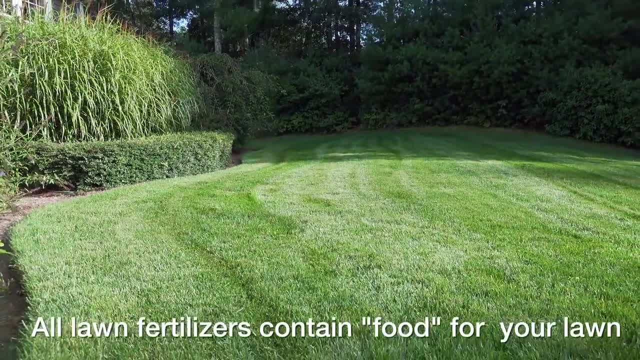 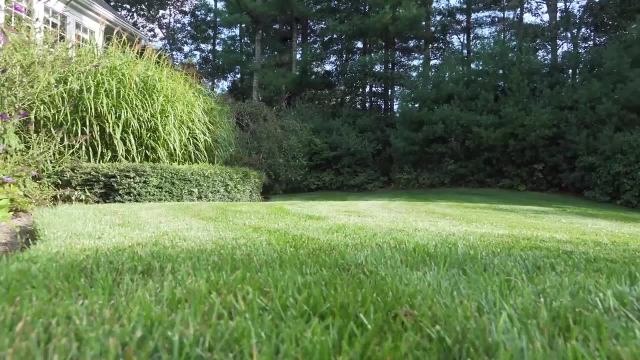 The key is that your lawn needs to be fed certain ingredients that every lawn fertilizer has, But does that mean that every lawn fertilizer is exactly the same and it doesn't matter what you buy? Well, the real answer is that it does, but not in the way you would think. 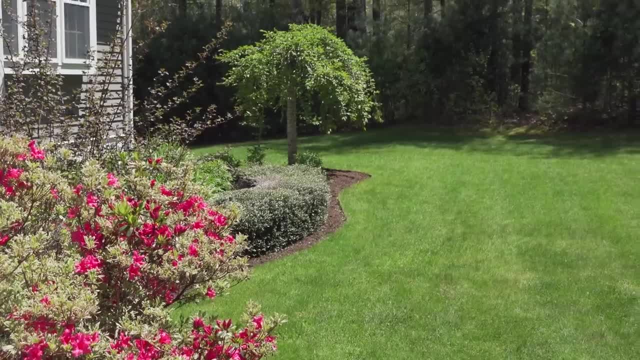 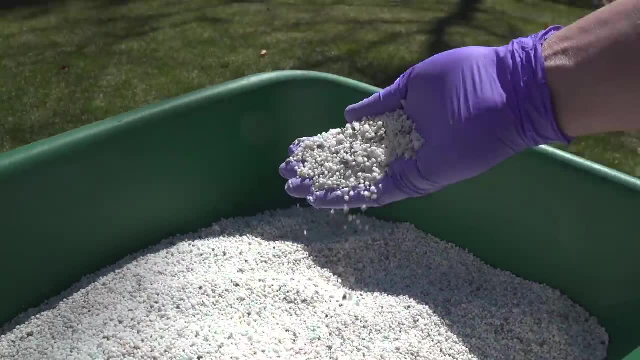 Now your lawn would grow without any added fertilizer, but it would never get that deep green color and it would probably not look the way you actually want. And that's my first tip: If you want your lawn to look its best, you want to fertilize it every four to six weeks during the growing season. 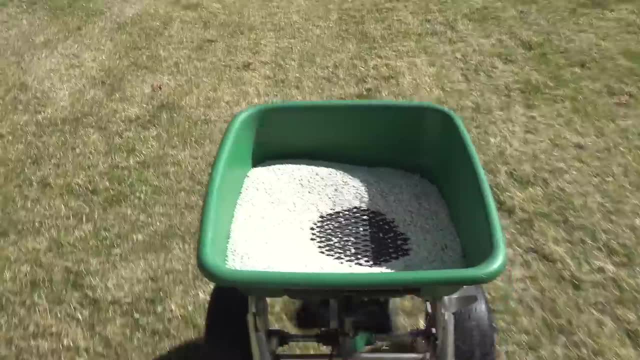 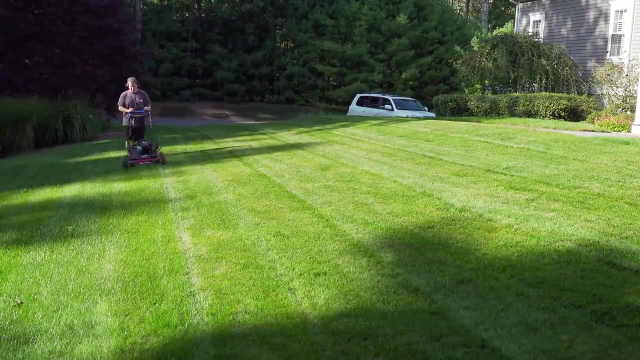 That's why getting an affordable lawn is so important And that's why a good fertilizer is key, because frequent feedings like that are going to make it look so much better all season long. But then what about the type of fertilizer you should use? 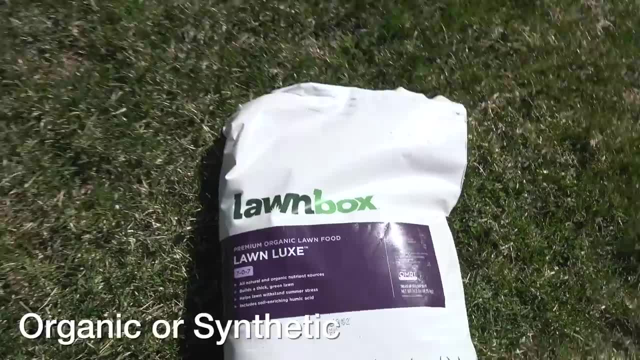 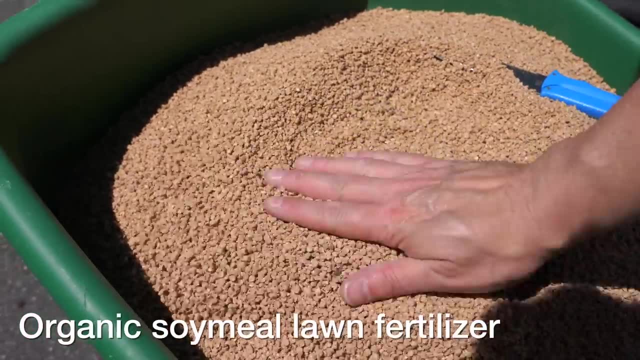 Well, all lawn fertilizers come in two categories. They're either organic or synthetic. Now, organic fertilizers are great. They're doing a lot better than they were in the past. They will give you a good looking lawn, but that will come at a higher price. 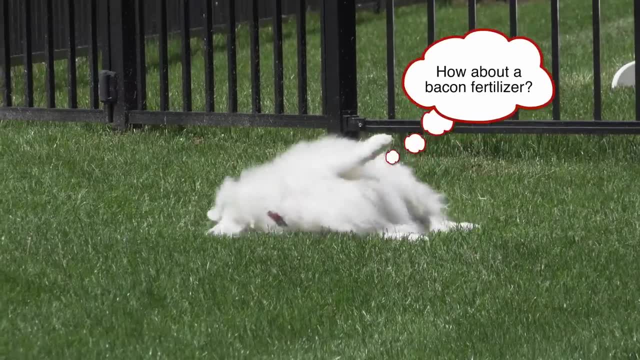 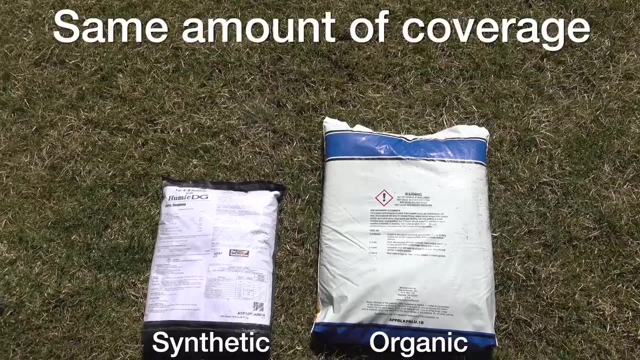 But for some people an organic fertilizer is the only way they're going to go. For most people, synthetic fertilizers will be a better choice and they're a lot more affordable. And because they're more concentrated, they're going to be in smaller bags and that means it's easier to handle. 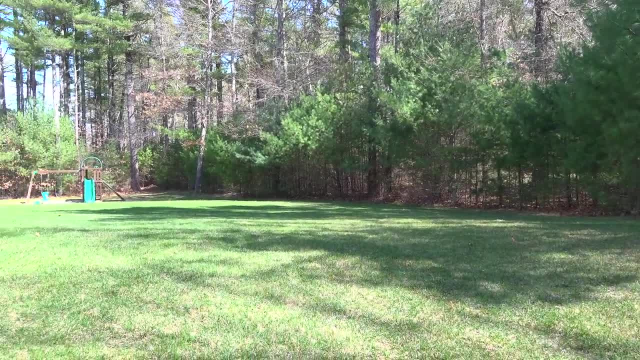 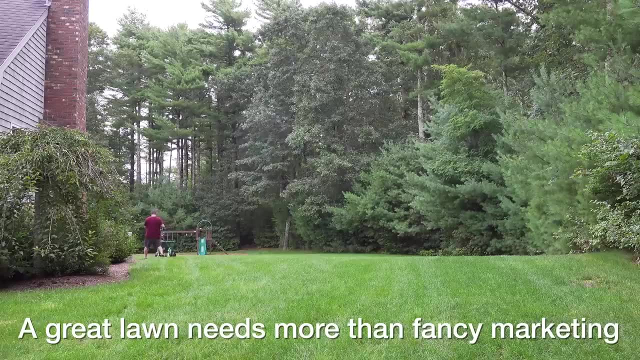 But then, which brand of fertilizer is going to be right for your lawn and which one is the best? Well, the real answer is: you can choose from a number of different brands, because it's less about the chemical formula and more about the pellets themselves. 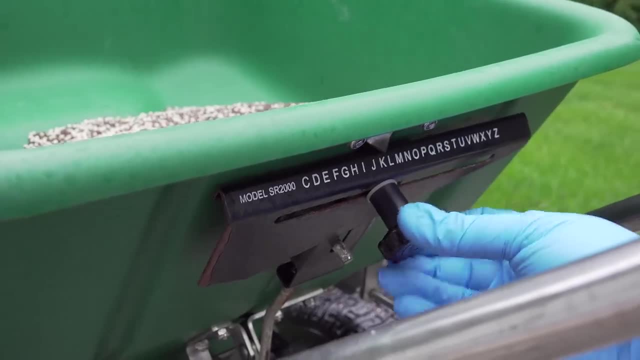 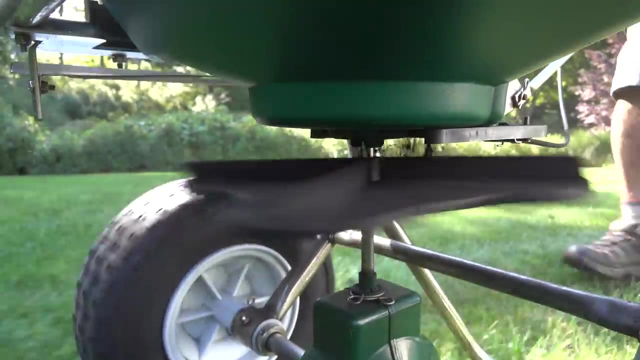 When you put a fertilizer down, two things need to happen. First, it needs to get on your lawn evenly, and second, it needs to be able to break down. Now, that might sound easy, but so many mixes get clogged in the bag itself. 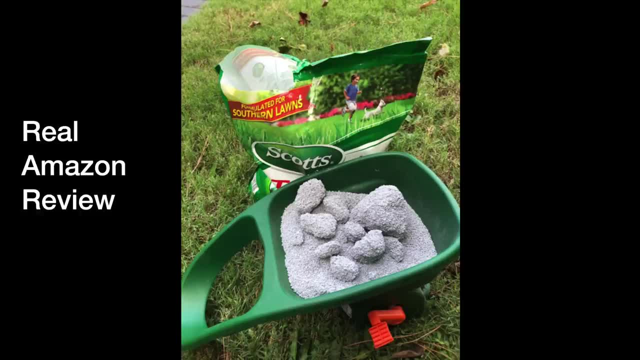 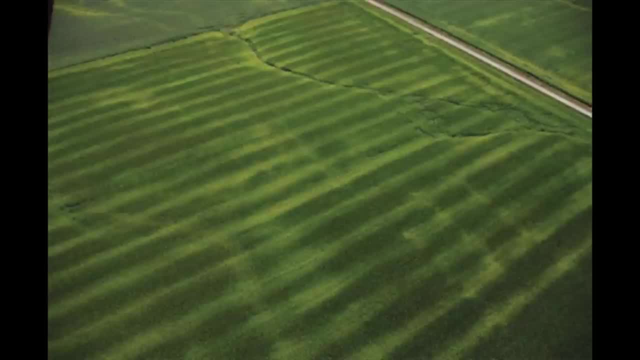 For years I used to use Scotts. Every bag would have a brick inside that would jam up in my spreader and I wouldn't notice it until I was halfway across the lawn. That meant uneven results, blotchiness, and it just wouldn't look good. and that's the whole reason. you're fertilizing your lawn to begin with. 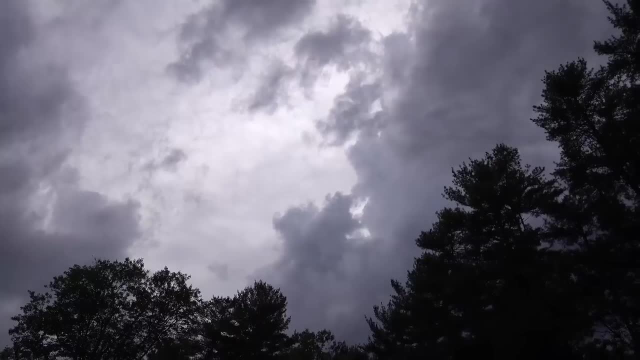 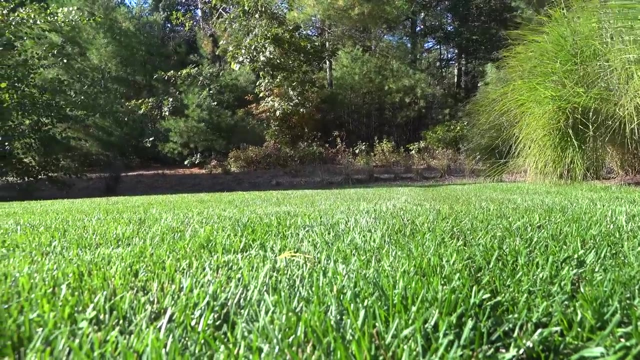 The other thing your lawn fertilizer has to do is break down over time. Now here in New England we get crazy weather: it rains a ton and then we won't see any rain for two months. And when it comes to those little pellets, if they're not designed to break down at a controlled amount, 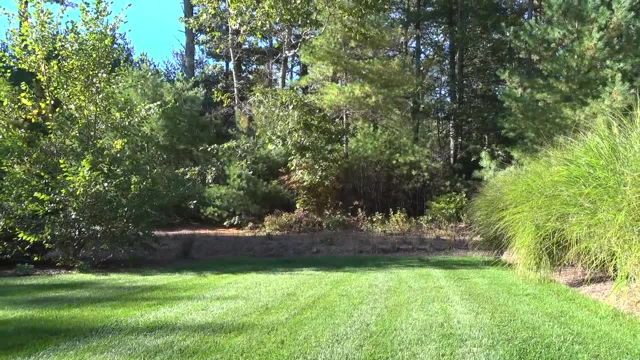 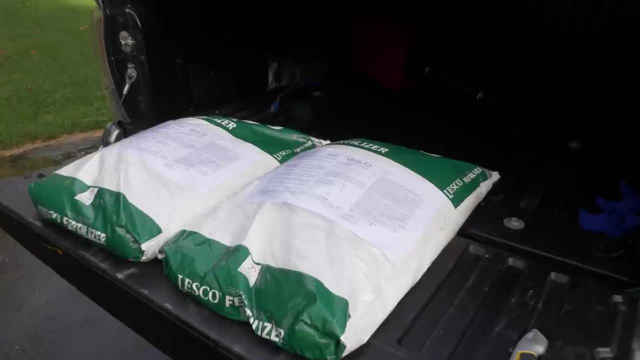 your lawn will either get too much food or too little, And I liked Lesko products a lot, but they had one problem: You can't really buy them anywhere. They don't sell online, and the versions they've got at Home Depot are not the same that the pros use. 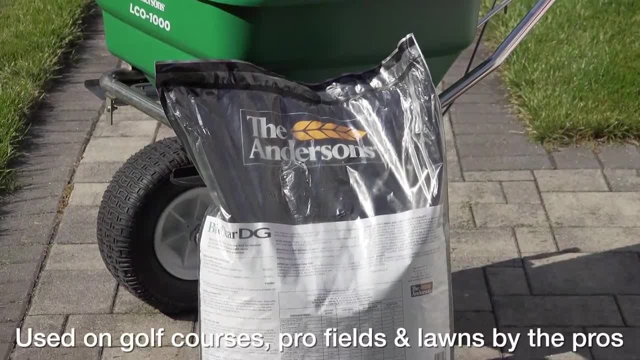 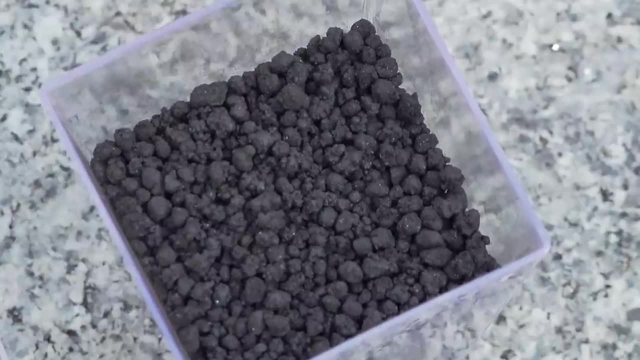 And that's when I got introduced to the company the Andersons. Now they make a lot of professional fertilizers but they've got a big difference. It's all about that pellet. It's so good, it's actually got a patent. 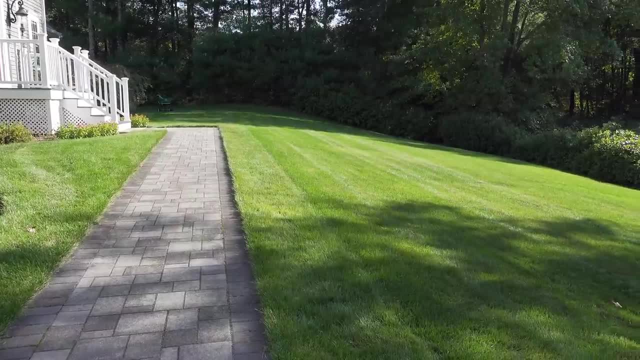 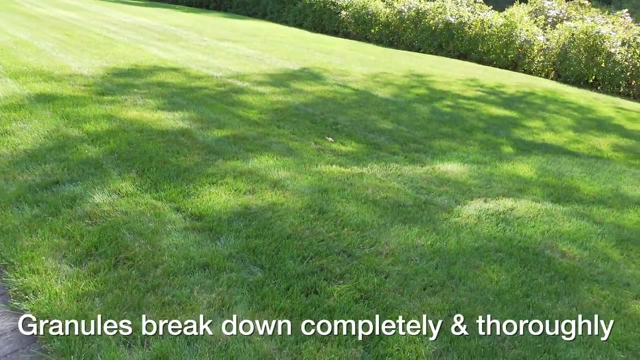 Now, this means less dust. for you, it's easier to apply because it's not going to clog in the bag or your spreader. But the best reason I like is that these pellets will dissolve at a very controlled rate, So if you're getting a lot of rain or a little, you're still going to get the right amount of fertilizer on your lawn at the right time. 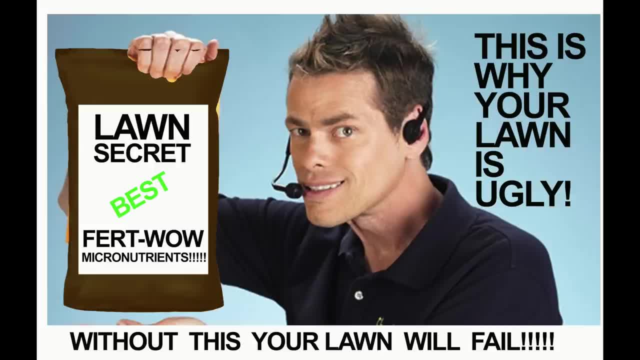 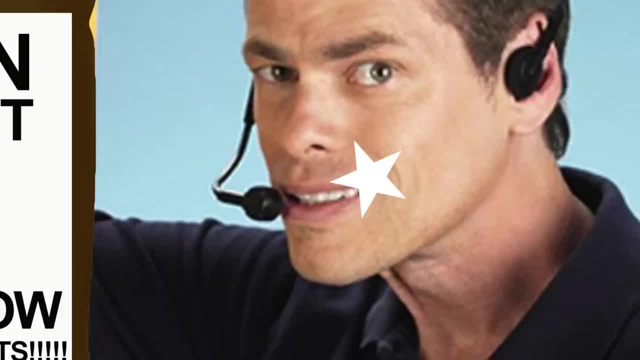 Well, you need to be aware there's a lot of new fertilizer companies that claim they've got a product loaded with things like micronutrients and supplements that your lawn absolutely needs. This is lawn fertilizer. These aren't craft beers or homemade apple pie. 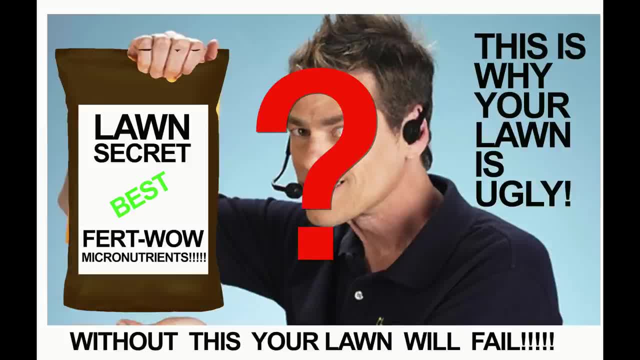 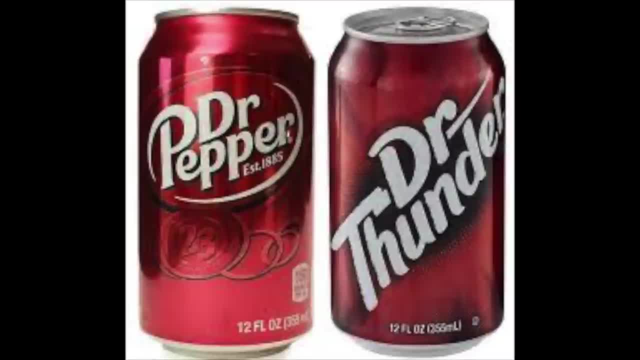 Fertilizers are chemicals, kind of like medications, and you want to get one that was made by a company who had the resources to know what they're doing. And the other trick is to just relabel an existing product, maybe change your thing or two, and now it's become the new miracle. 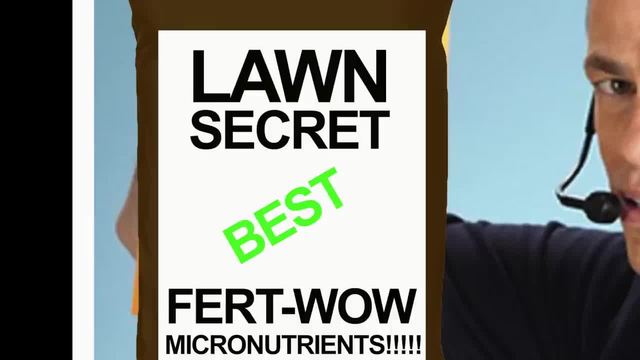 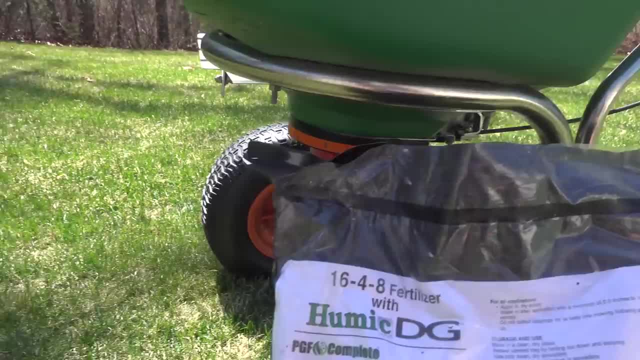 The only use for these niche fertilizers is to make the people a lot of money who are trying to sell them to you, Because the best fertilizer is the one that you can actually afford and it works on your lawn. Now, for me, I use the Andersons PGF Complete product. 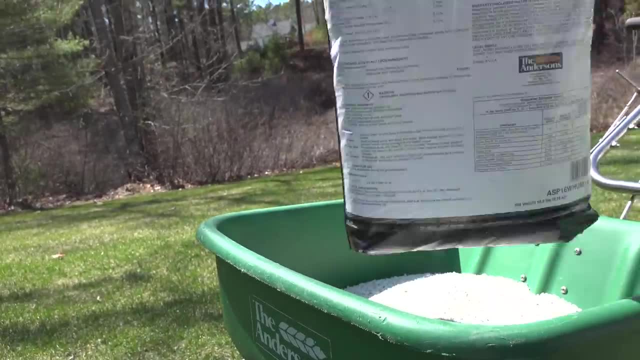 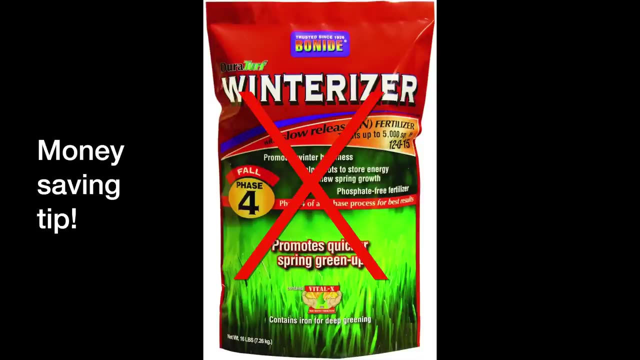 It's affordable, you can order it online and it's really easy to apply, because they've got those pellets that actually dissolve at a controlled rate. And here's another tip: that's great. It's going to make your lawn care easier and save you money. 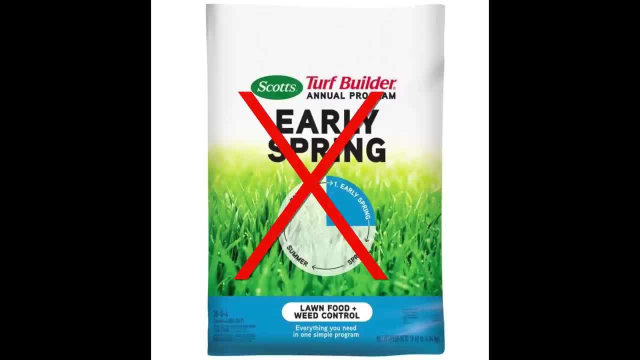 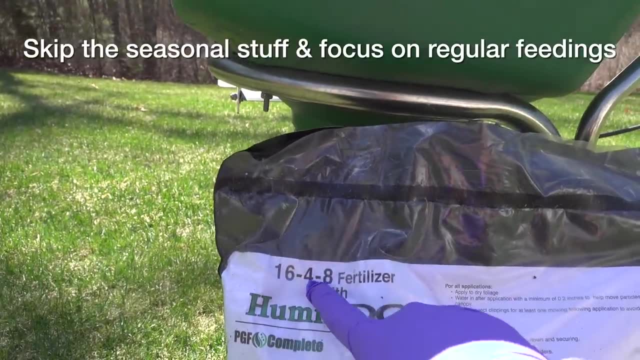 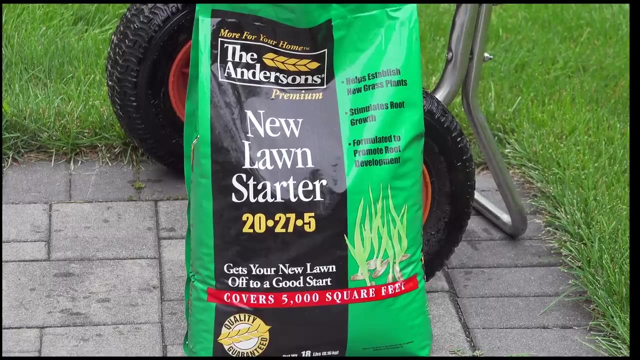 You don't need to bother with winterizers, fall and spring fertilizers, Just buy one fertilizer like this and use it all season long. I've never used those specialty fertilizers and have had nothing but good results, And the only exception is I'll use a starter fertilizer if I'm going to be putting down seed or if I'm overseeding my lawn.